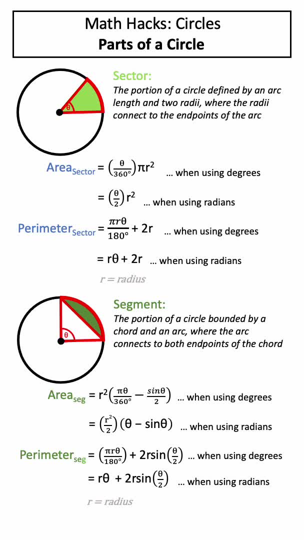 And similarly, the area and perimeter can be calculated using the formula shown here. they're shown here.